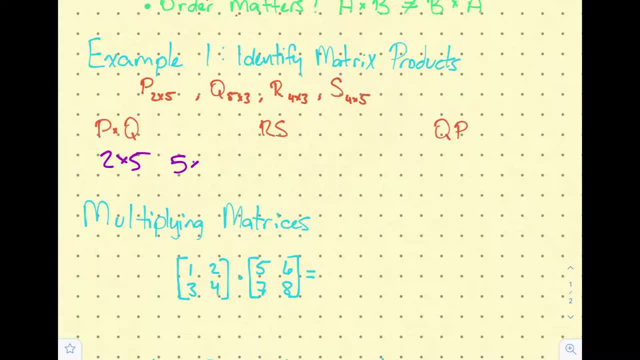 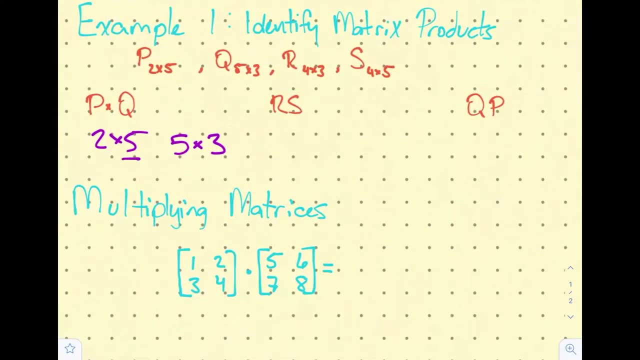 5 by 3 matrix matrix, Because the number of columns in our first one- 5, matches the number of rows in our second one. we are allowed to multiply these together. We will end up with a 2 by 3 matrix. as a result, Let's check out R times S. R is a 4 by 3.. S is a 4 by 5.. So if we 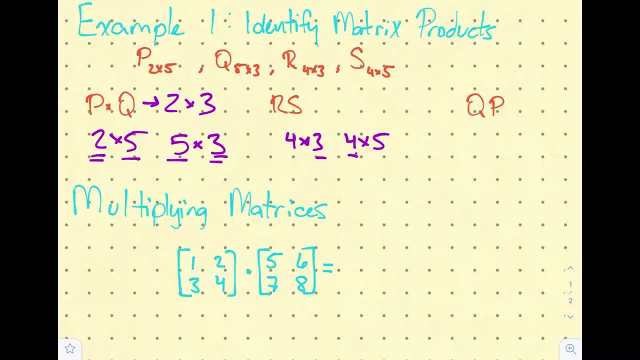 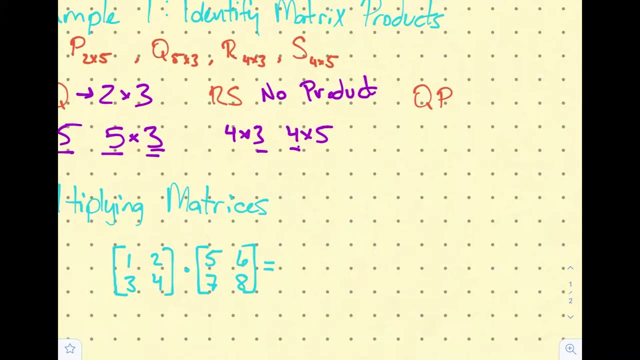 check. the number of columns in R does not match the number of rows in S, so we are not allowed to multiply them together. There is no product. Alright, let's check out one more pair We talked about. we already looked at PQ. Let's look at QP. Q is a 5 by 3 matrix, P. 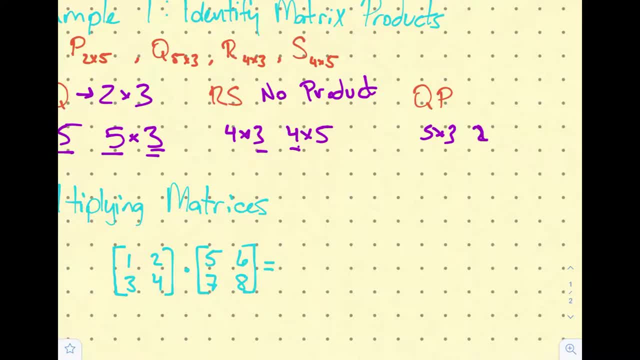 is a 2 by 5 matrix And again, the number of columns in Q does not match the number of rows in P, so I cannot multiply them. There is no product. So now that we've checked if we are allowed to multiply two matrices together and what, 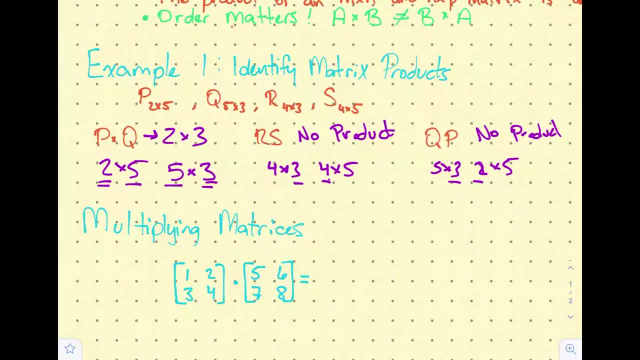 kind of matrix we'll get as a result. Now let's go through the how to multiply and why the number of columns has to match the number of rows. And I want to be very clear: The product of this is not 1 times 5,, 2 times 6,, 4 times 8.. Cryptos will, because they have 4 rows into them And that is clearly why they will multiply the number of qualité. get into the life number 3.. 9 times 2 is not the number of rows, And 3 times 4.. 7 times 5 equals. 5 and 12 times 7 is how many rows that we get. So these are different. Now, we'veulares are 2016 products And they are marryable, and they are not the number of rows which, at one time in the other world that's not increase sometimes what we're calling them bad kids. 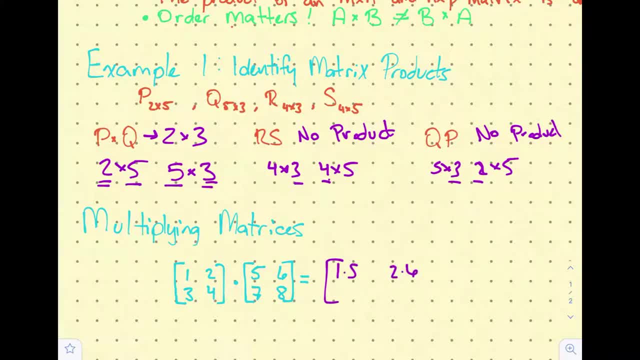 2 times 6,, 3 times 7,, 4 times 8.. That is not how matrix multiplication works. Instead, for each element, I'm going to take this row and multiply it by this column. I'll have 1 times 5 plus 2 times 7.. 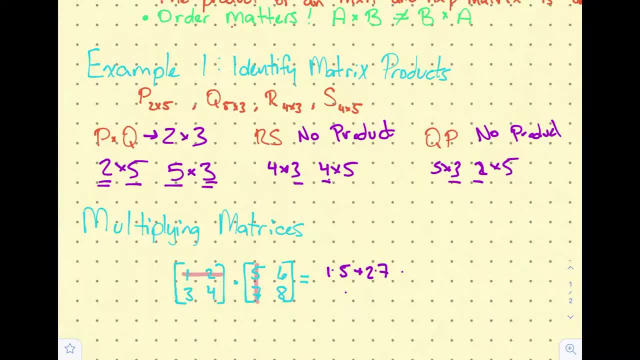 And because this is the first row, first column, it's the element that goes in the first row, first column And then we just work down the line. Since I'm done with that column, I'll move to the next one. The first row, second column will be 1 times 6 plus 2 times 8.. 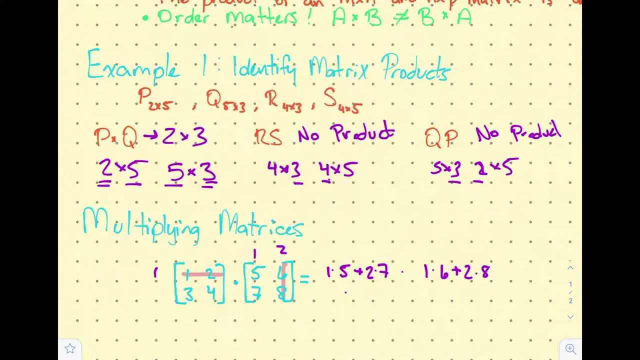 And now that I'm out of columns, I'll move down a row. in my first matrix We're going to take the second row and we're just going to repeat. I'm going to multiply by the first column 3 times 5 plus 4 times 7.. 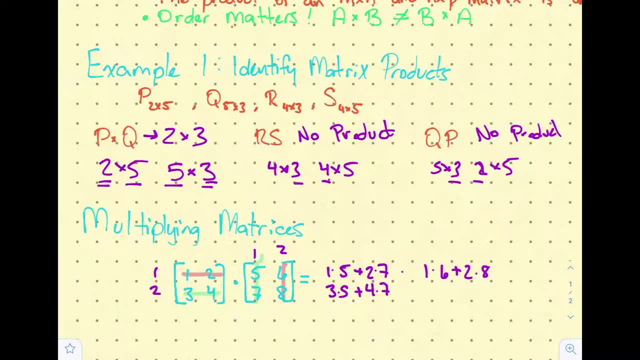 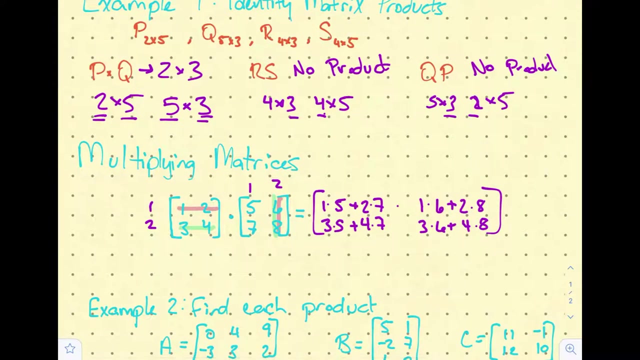 And once I'm done I'll move over to the next row. 3 times 6 plus 4 times 8.. And then we can evaluate: and that is our next or that's our product. So the product of these two matrices is 19,, 22,, 43.. 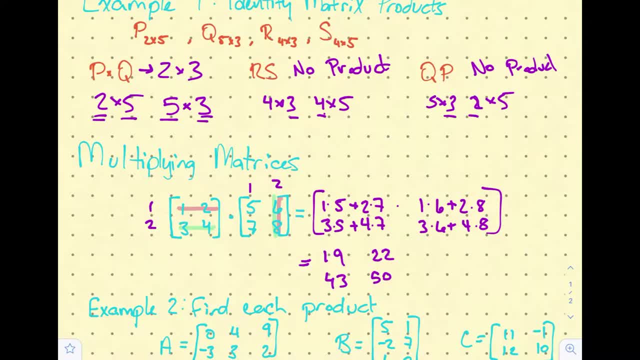 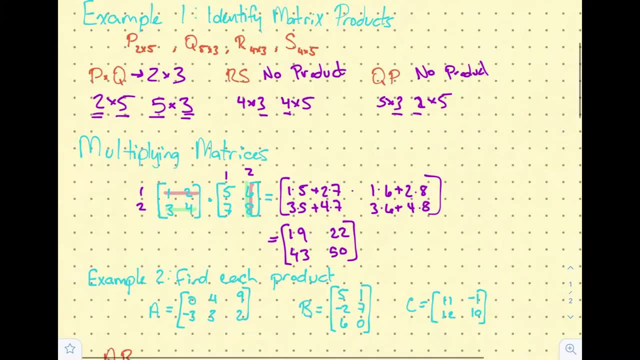 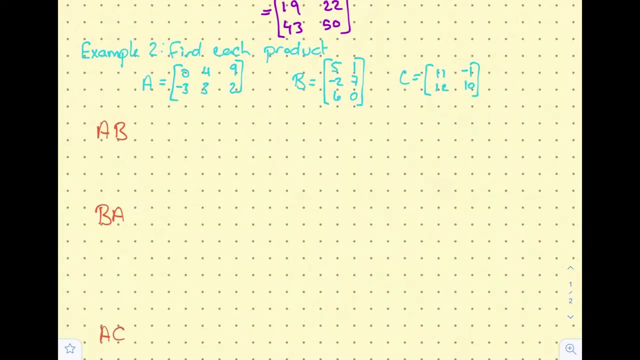 That is the product of these two matrices. So let's do another couple of multiplications together. For each one, we're going to determine if we're able to multiply, We will determine the size of the result and then we will actually multiply. 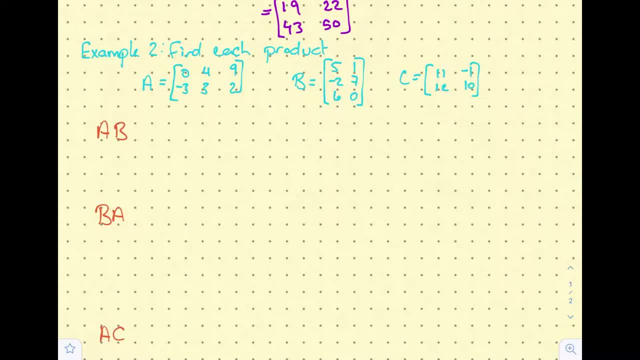 So first, A times B, A is a 2 by 3. matrix B is a 3 by 2.. So because we are allowed to multiply, we will end up with a 2 by 2 matrix as a result. So just remember, we're going to take each row, multiply it by each column. 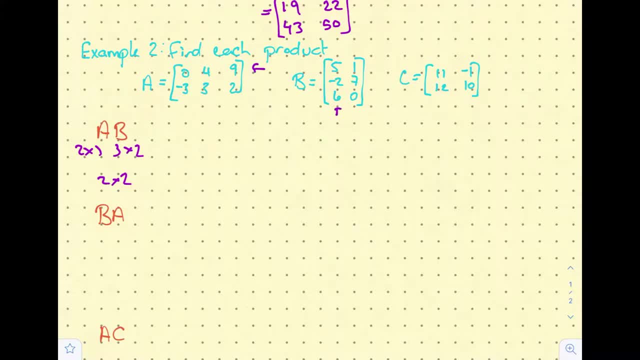 So our first row, first column element is going to be 0 times 5 plus 4 times negative, 2 plus 9 times 6.. Our first row, second column- if I just move my arrow over to the side, one spot. 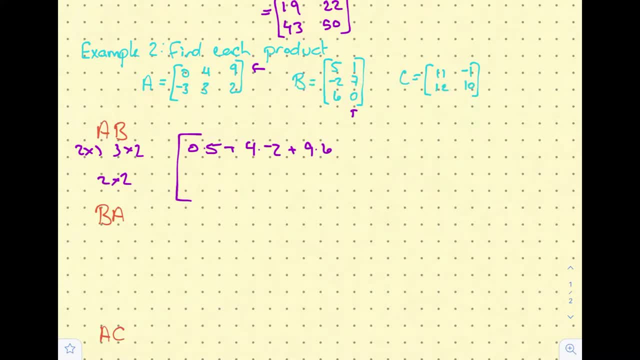 it is going to be 0 times 1, plus 4 times 7, plus 9 times 0.. And now I'm going to repeat, but with the second row. So I have negative 3 times 5.. Plus 3 times negative 2, plus 2 times 6.. 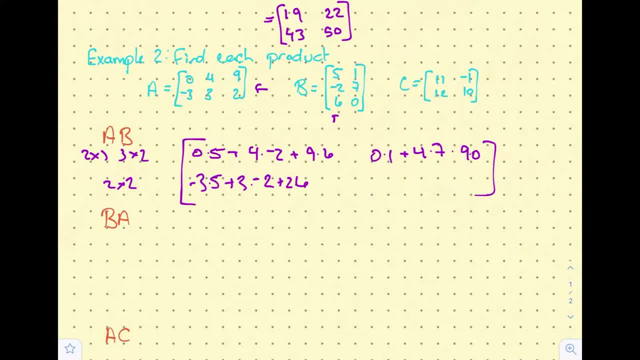 And then, if I move over to the next column, I have negative 3 times 1, plus 3 times 7, plus 2 times 0. And then evaluating this out will give me my resulting matrix. So I'm going to multiply this by 0.. 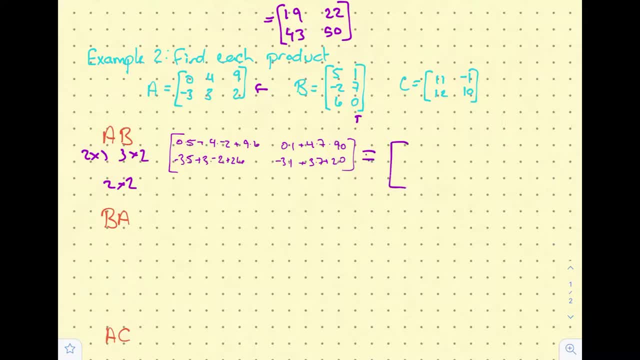 0 times 5 is 0.. 4 times negative: 2 is negative 8.. 9 times 6 is 54.. 0 plus negative: 8 plus 54 is 46.. In the next column, 0 times 1 is 0.. 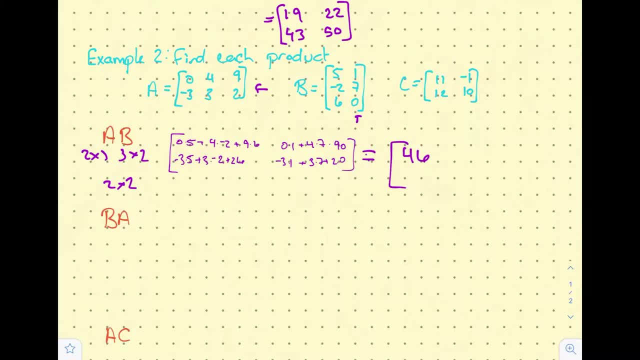 4 times 7 is 28.. 9 times 0 is 0.. 0 plus 28 plus 0 is 28.. 0 plus 28 plus 0 is 28.. And carrying down the line, see that's negative 15 and negative 6 is negative. 21 plus 12 is negative 9.. 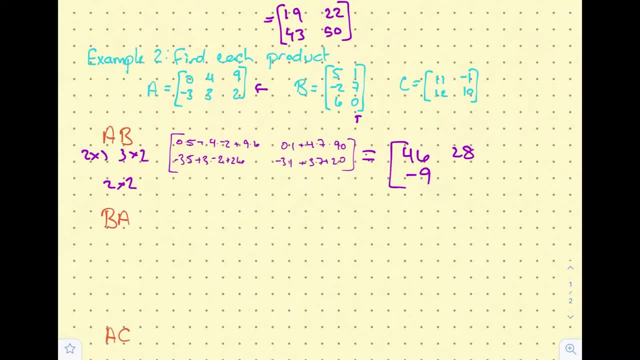 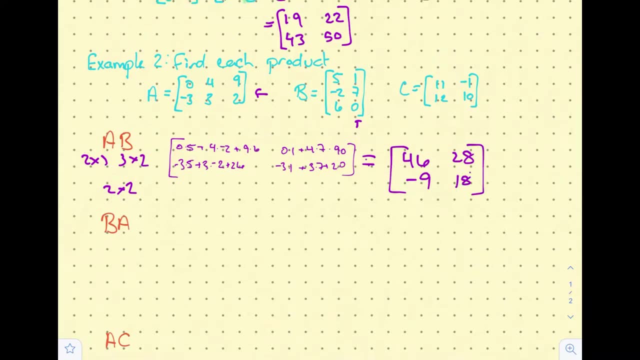 And negative: 3, 21 and 0 is 18.. All right, And one more time to demonstrate That order matters. Let's find B times A. B is a 3 by 2 matrix And A is a 2 by 3.. 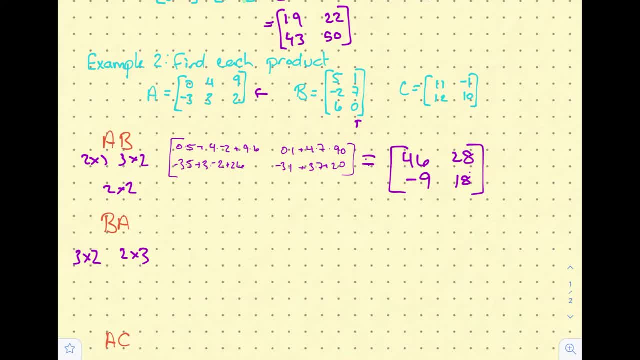 So we are allowed to multiply them, But we will end up with a 3 by 3 matrix. as a result, I need to take a row from B multiplied by a column from A, So we'll have 5 times 0.. 0 times 0..